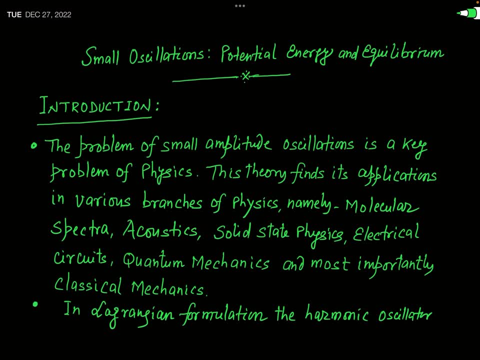 advanced concept of a small oscillations. in fact, you know that this problem of a small oscillations- when you say small oscillation, that means the oscillation or vibration with a small amplitude- this is just a key problem of physics. why this problem of a small oscillation is called key problem of physics? because 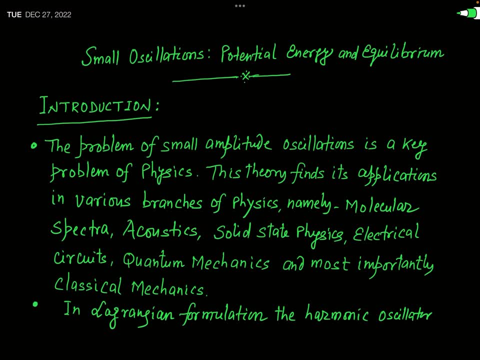 you know that the theory of a small oscillations finds its applications in various branches of physics and definitely you have been encountered with this problem while studying the different branches of physics, as, for example, you can say that when you study the, the molecular spectra, then we study their rotational vibrational spectra and the concept. 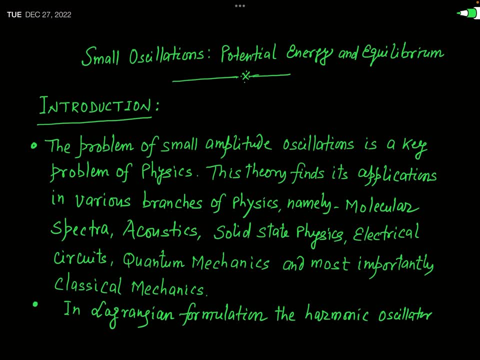 of linear harmonic oscillator is in fact used there. okay. similarly, in acoustics we find the problems on a cost, on a small oscillations in solid state physics, while studying the vibration of atoms in solid, you face this problem and in case of electrical circuit, you study the LC oscillation. okay, in quantum mechanics this is a very important problem. 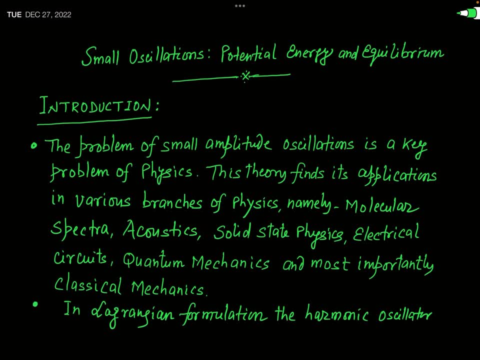 while studying the quantum dynamics and the problem of linear harmonic oscillator, you in matrix formulation of quantum mechanics and several you in matrix formulation of quantum mechanics and several other places, you find the problem of a small oscillation and, most importantly, in classical physics you have been studied the problem of a spring mass system, simple pendulum, bar pendulum. 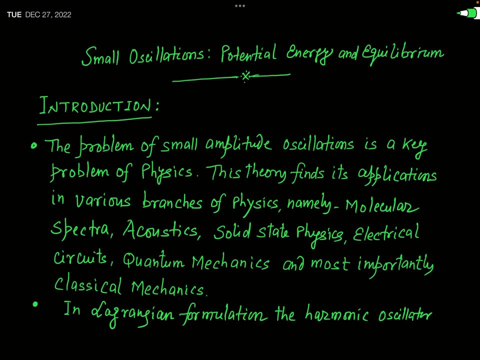 compound pendulum, caters pendulum, and so and everywhere you have faced this problem of a small oscillations. so this, this problem of a small oscillation, is very important and its concept is a somewhat- it you can say its concept is somewhat tedious, but when you will watch my videos on this, 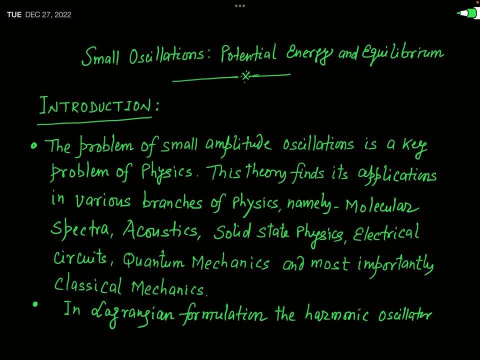 chapter. in of this chapter, the advanced concept of oscillations will be definitely cleared to you. okay, in fact, you can see that the concept of oscillations is somewhat tedious, but when you will watch my videos on this chapter, the advanced concept of oscillations will be definitely. 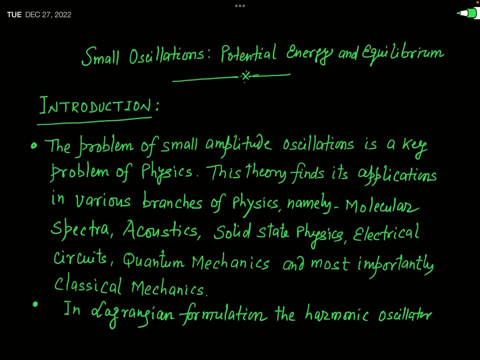 treated here, as I stated many times, by an imagine that such a consequence. but what we do have, if you knowлично, I think they were crude- me election with this concept, yet noticed Bauk, seventy be told, which is commitment to the system, as I said. so you may have understood the function. 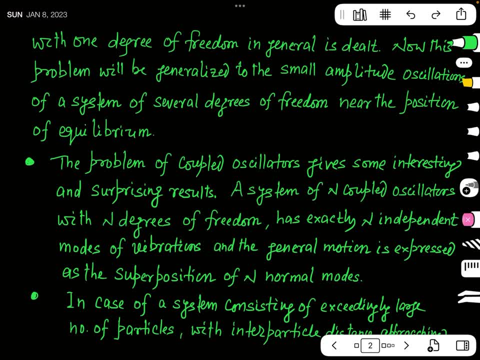 based on the'- what was the expression? and the q, and of freedom. okay, but in this chapter we are going to generalize that problem. it means it means we have to generalize the problem in such a way that the degree of freedom will be not limited to one, but we will see the oscillation of such a 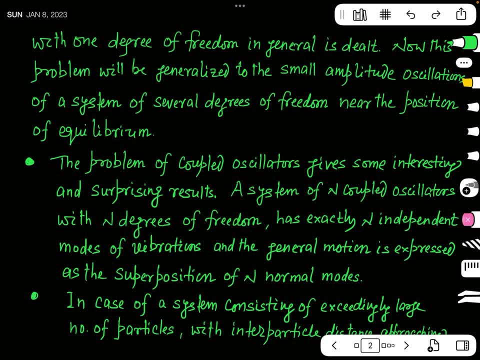 system which has actually several degrees of freedom near the equilibrium position. okay, and so this? you can say that we are going to discuss the theory of a small oscillations in general form, where we will deal with the harmonic oscillator problem not of only one degree of freedom, but several degrees of 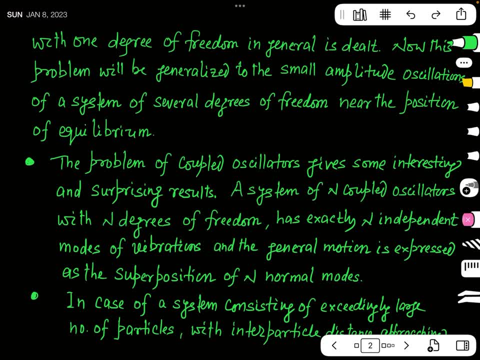 freedom. okay, and that's why we will get some new idea, new concept, new results. okay. in fact, when we will study this chapter, you will see that we will solve the problem of coupled oscillators. while studying the problem of coupled oscillators, you will see there will be. 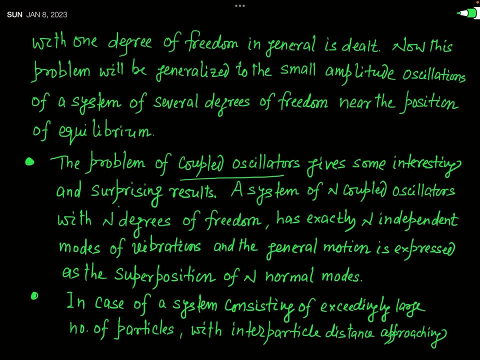 some very interesting and surprising result. okay, when we will solve such problem, you will get that there are very interesting and surprising results. okay, if you consider that there is a system of n coupled oscillators with n degrees of freedom, then you will find that there will be exactly n independent modes of vibration, or you can say n independent. 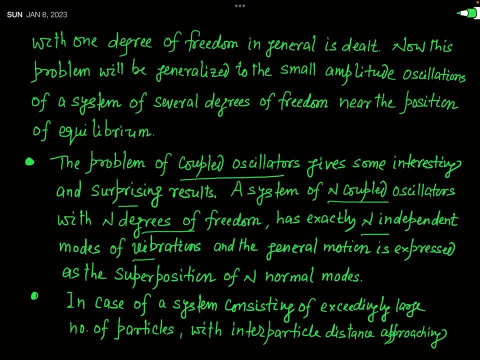 normal modes of vibration, okay, and the general motion will be just the super, sorry superposition of n normal modes. okay, in fact, when you will consider a system consisting of a very large number of particles, exceedingly large, or you can say infinitely large number of particles, such that the inter particle 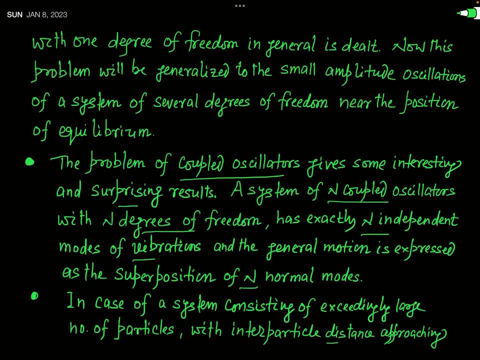 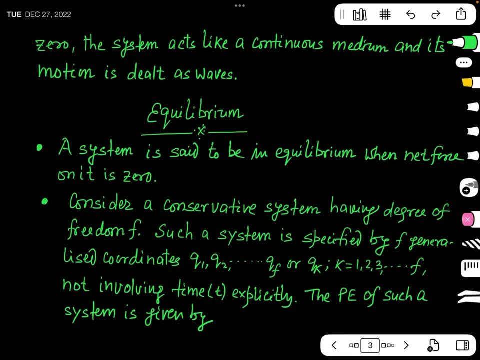 separation or inter particle distance is almost equal to zero, then such a medium is treated just like a continuous medium and in fact, in that condition, while discussing the oscillation, we will discuss it just in terms of waves. so the idea of waves is also developed from the idea of vibration. in fact, in that condition, our system, in our system, 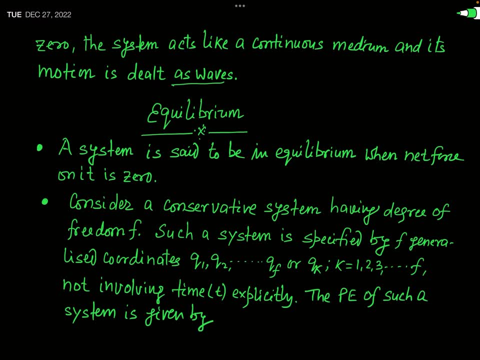 the particles are distributed just in a continuous fashion, in a continuous manner, and then that vibration can be described in terms of waves. okay, now, any oscillator vibrate or oscillate about equilibrium position. so, before a starting this very chapter, i would like to explain the concept of equilibrium. so in this introductory, 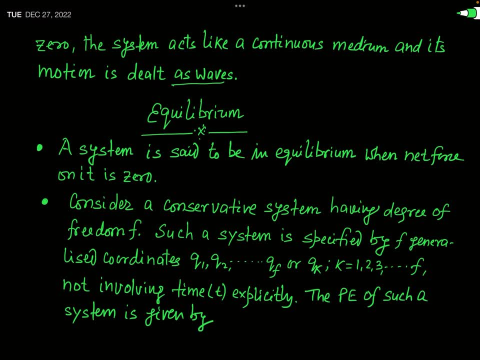 lecture, or the first lecture on a small oscillation. i am just going to explain what is equilibrium and what is that. why we are going to talk about equilibrium and why we are going to study equilibrium- because i have told you that the oscillation always takes place about. 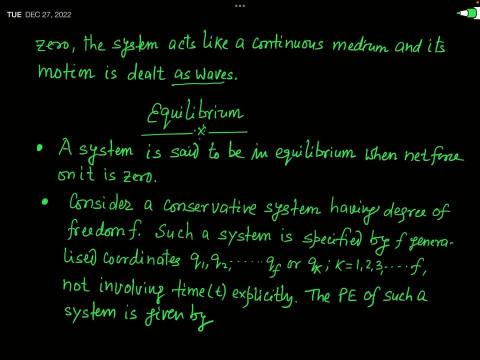 the position of equilibrium. so definitely, the concept of equilibrium must be in your mind to understand the concept of oscillation. okay, this equilibrium is also not new for you, because you have definitely studied the concept of equilibrium, uh, in your lower classes. so thus, just toidos, it became scenery focused on the concept of equilibrium. so the installation. 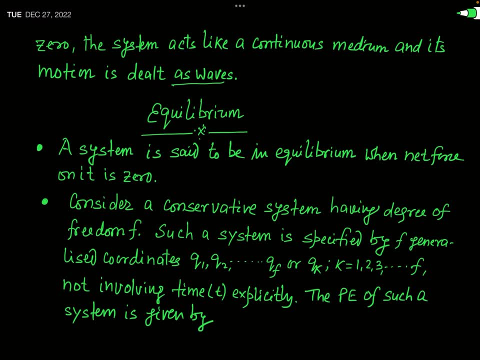 of the system in the Тыnö r system in the. this is just a revision so that you will not find any difficulty in understanding the concept of a small oscillation. in fact, when you say that there is a system which is in equilibrium, what does it? 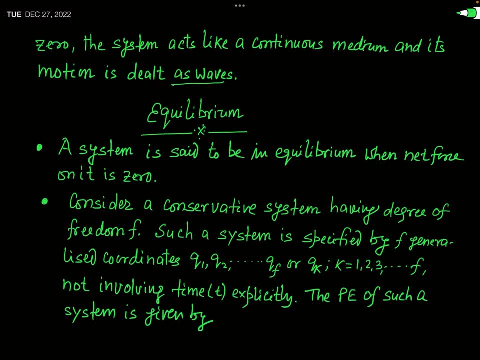 mean. a system in equilibrium means that the net force or the resultant force on the system is zero. in other words, you can say that if a resultant force on a system is zero, then such a state of the system is called its equilibrium state. okay, net force must be zero on the system to be in equilibrium. 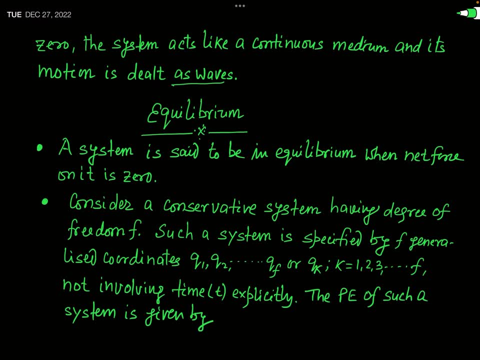 state okay. so in fact, this concept of equilibrium can be understood in terms of potential energy because, you know, in the advanced classical mechanics, where we talk about the hamiltonian mechanics and lagrangian mechanics, we do not talk in terms of force, but we always talk in terms of energy. so the concept of 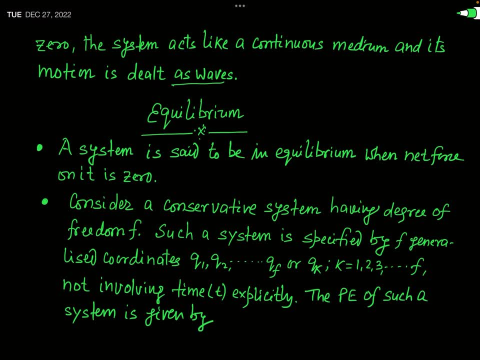 equilibrium should be also in terms of energy. in fact, for a conservative system, the concept of equilibrium can be described in terms of potential energy of the system. you know that a conservative system is always associated with a potential energy corresponding to the conservative forces. okay, so to understand the idea of equilibrium, let us consider a conservative system and this. 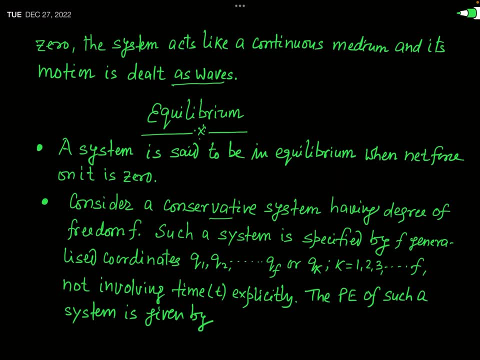 conservative system has, let us say, degree of freedom F. F is the number of degree of freedom of our conservative system and, as you know, if f is the number of degree of freedom, definitely the number of independent variables or the number of generalized coordinates to specify the configuration of the system must be equal to f, and we denote those. 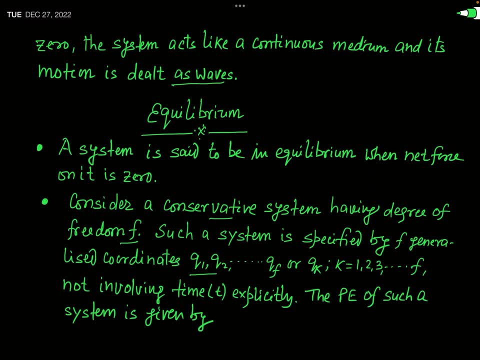 generalized coordinates by the symbol q1, q2, q3, so on qf. so you can say that these q1, q2, so on qf, are that generalized coordinates of this conservative system. okay, in brief, you can also say that the generalized coordinate of this conservative system are qk, where k is one, two, three. 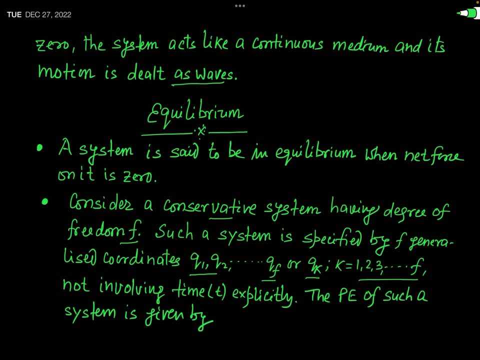 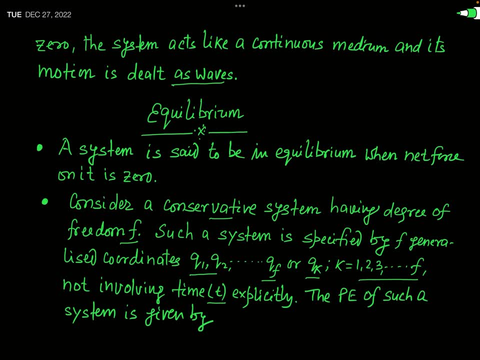 It means you are considering the stationary system time independent. okay, In fact, if the potential energy of such a system can be expressed, definitely that potential energy, as depends on the configuration of the system and the configuration of the system, is described in terms of these generalized coordinates. 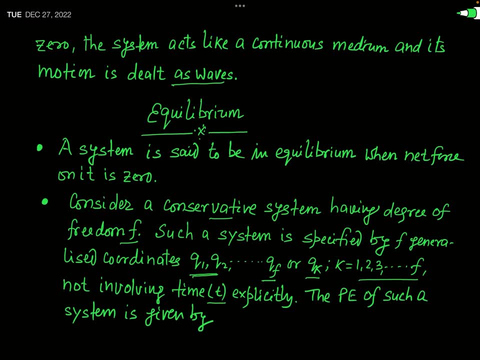 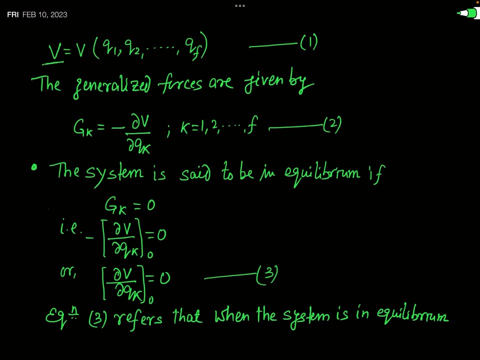 So you can definitely say that the potential energy of such a conservative system will be just a function of these generalized coordinates. Okay, So you can write that the potential energy function of this conservative system is just equal to v of q1,, q2, so on qf. okay, 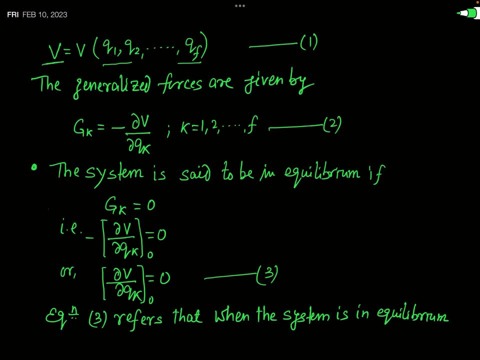 And, as you know, that the generalized forces are simply the negative of the partial derivative of potential energy function with respect to the generalized coordinate. or, in other words, we say that the generalized force is the negative coordinate, It is the gradient of the potential energy function. 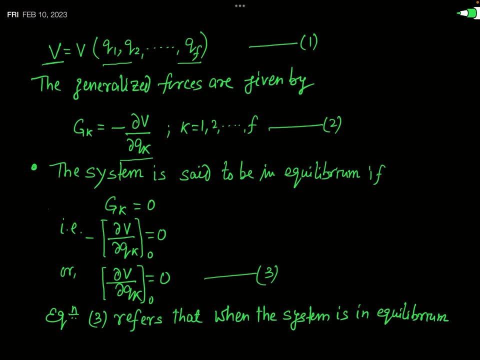 So if you write the kth component of the generalized force by the symbol gk- this gk represents the kth component of generalized forces- then gk is equal to minus del v by del qk. You know it. In the very beginning of Lagrangian formulation we have defined the several generalized quantities. 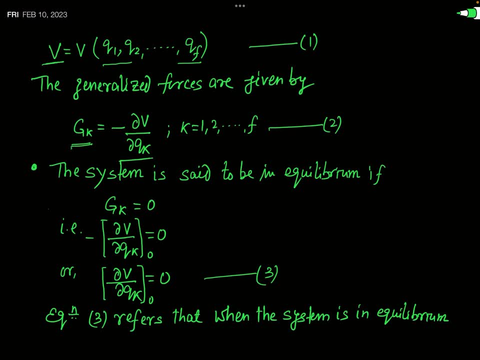 and there you will find, in my video, the concept of generalized force, and that generalized force is defined like minus del v by del qk. Okay, Now, as in the beginning, I have told you that any system is said to be in equilibrium when 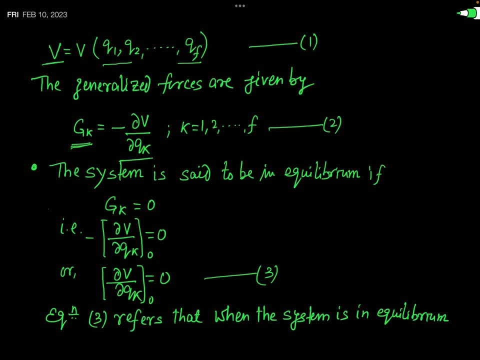 the net force on it is equal to zero. So if net force will be zero, Okay, Each and every component of the force will be zero. If net force is zero, then each and every component of the force will be zero. For example, let us consider the not generalized force, but in general, the force vector. 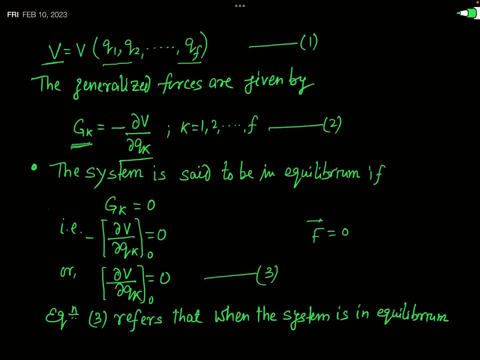 And you say that this force vector is zero And in the 3D space you write this force vector as fxi plus fyj plus fzk. You write it And this is equal to zero. You know, if fxi plus fyj plus fzk is zero, it is possible only when all these components are separately equal to zero. 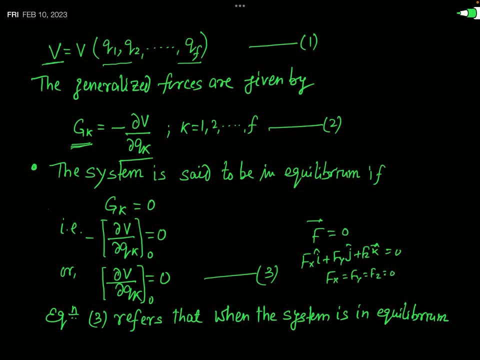 Only then this force will be 0.. So if our system is in equilibrium, then in accordance with the definition of equilibrium, we can say that the kth component of the generalized force, gk, will be equal to 0. It means g1, g2, g3- all will be equal to 0. But as we know that, 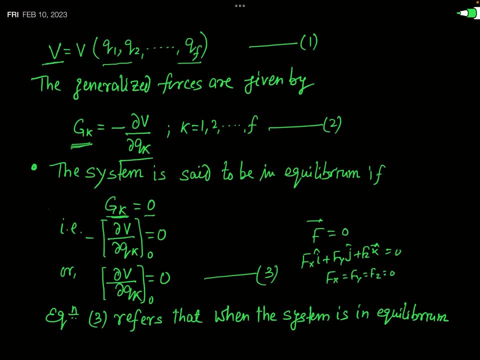 this gk is equal to minus del v by del qk, and at the equilibrium position this should be equal to 0. So we can say that minus del v by del qk is equal to 0 at the equilibrium position. Here this subscript 0 actually refers the equilibrium position. This subscript, which 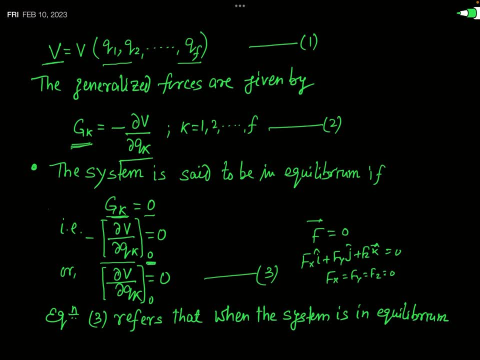 I have mentioned here, outside of the bracket, that actually represents what That represents, that we are talking about the value of this minus del v by del qk at the equilibrium position, and at the equilibrium position this will be equal to 0.. Now, since in RHS there is 0, so you can. 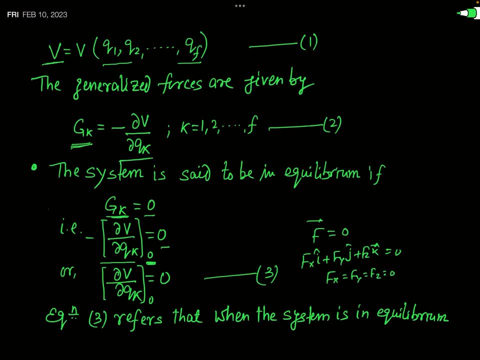 omit this minus sign and simply say that this del v by del qk at the equilibrium position is equal to 0.. So this is the condition for equilibrium in terms of potential energy function. So whenever we have to test that any position or any configuration or any state of the system is equilibrium, 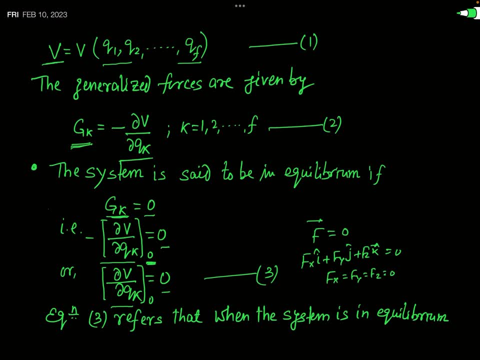 state or not what we will check. We will simply find the derivative of partial derivative of this potential function with respect to the generalized coordinate. At that point we can say that the equilibrium position is equal to 0 at the equilibrium position, And if that will be equal to 0, you can say that the system is in equilibrium. This is 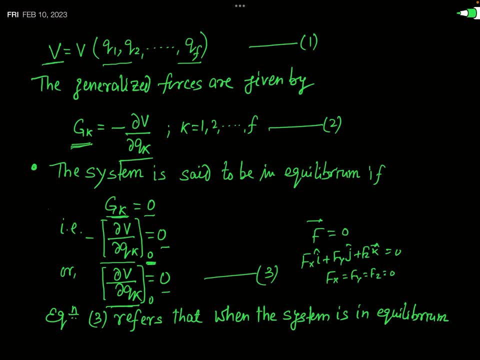 the mathematical condition for equilibrium in terms of potential energy function. But you know that if del v by del qk at the equilibrium position is 0, what does it mean? It means at the equilibrium position the potential energy function will be extremum Potential. 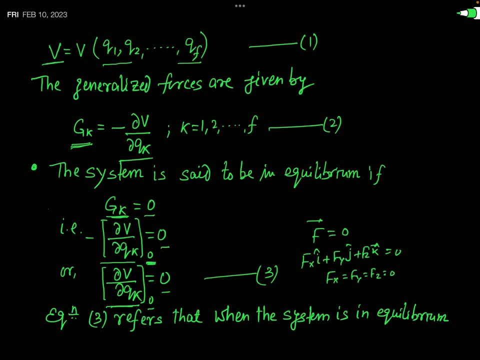 energy function of the system will be extremum. When you say extremum, what does it mean? It means v is either minimum or maximum, or stationary. When you say stationary, that means constant. It means at the position of equilibrium or in the state of equilibrium. 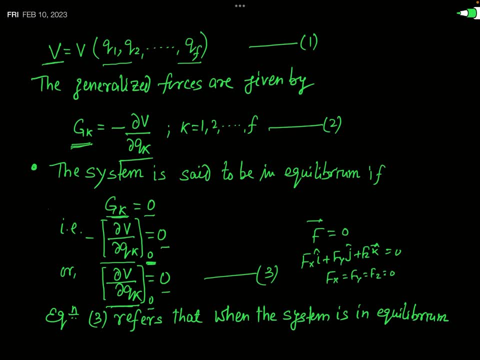 the system has either minimum potential energy or maximum potential energy or constant potential energy. Constant potential energy means when you will change the state of the system slightly, or position of the system slightly, there will be no change in potential energy. So in these three conditions the system will be said to be in equilibrium. So for equilibrium, 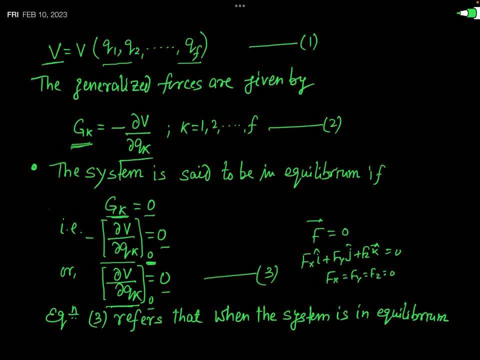 what is the condition? Condition is potential energy function of the system must be extremum. When you say extremum, extremum means the equilibrium of the system. When you say extremum extremum means the equilibrium of the system must be somewhere between minimum and maximum. 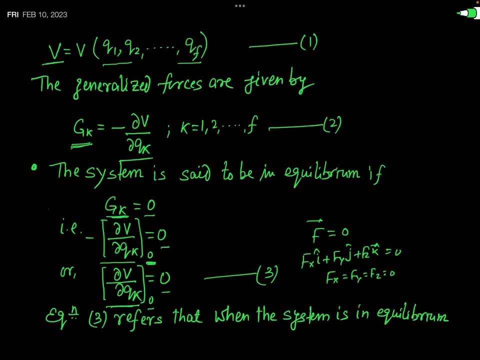 So it is either minimum or maximum or stationary. When you say minimum, it means that the cell does not move. When you say extremum, you will say extreme is either minimum or maximum or stationary. If you plot a graph, let us say between the generalized coordinate Qk. 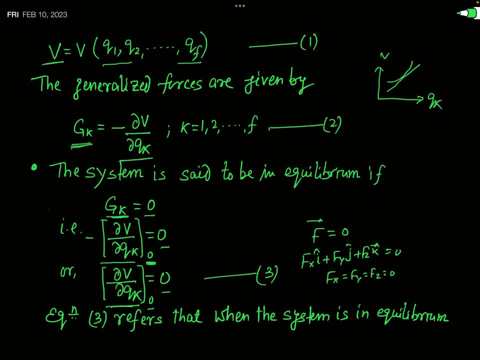 and v. let us say that this is our curve. Then del v by del qk means what, At any position, represent the slope of that point, slope of the curve at that point. So you can also say that if the slope of the V versus QK curve, V versus QK curve, which 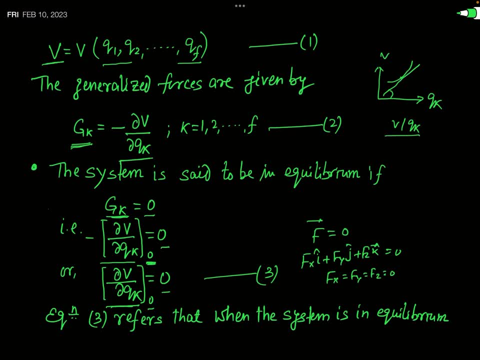 is actually called potential energy curve is equal to zero, at that point the system is in equilibrium. You can say: if the slope of the potential energy curve is zero at a particular point or in a particular state, then the system in that state is called equilibrium state or 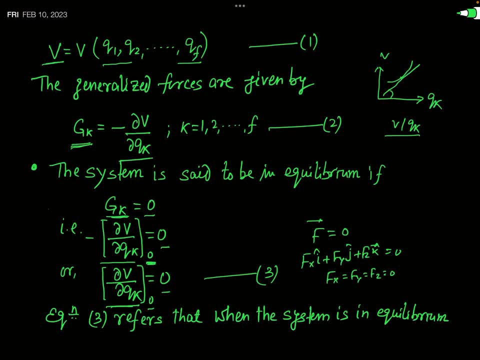 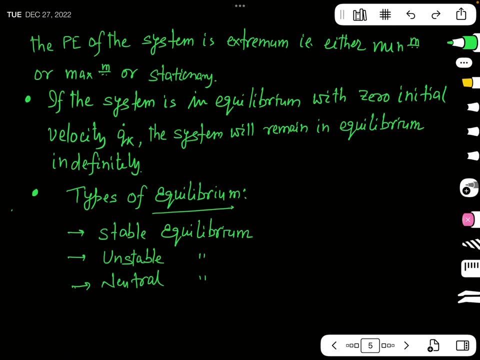 you can say that state of the system is the equilibrium state. So you can see- I have actually mentioned this fact here- that if the system is in equilibrium and potential energy of system is extremum, that is either minimum or maximum or stationary. Now let us see that this position, let us say O, is the equilibrium position of our system. 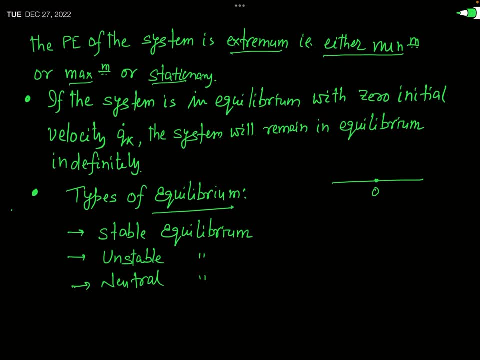 So if the initial velocity of our system is zero, then if the system will be at the equilibrium position, it will be permanently at that point, It will be never displaced. Okay, So at the equilibrium position the system remains indefinitely, for long time, for all time, if the initial velocity of the system is zero or if we do not displace the system. 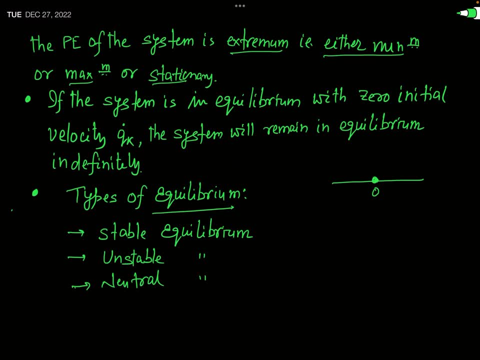 or do not disturb the system, then the system will permanently remain at the equilibrium position. Okay, So I hope you have understand what is the idea of equilibrium In terms of the potential energy function, the main thing is only two. First of all, you can say that the state of a system, when net force on the system is zero, 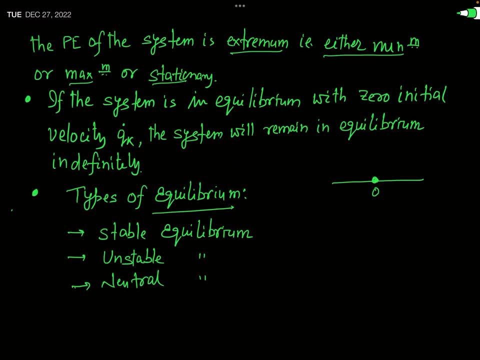 that state is called equilibrium state. and if net force is zero, then the negative of the gradient of the potential energy function should be zero, and that means the potential energy function of the system must be external. Okay, So if the system is in equilibrium state, and if the system is in equilibrium state, then 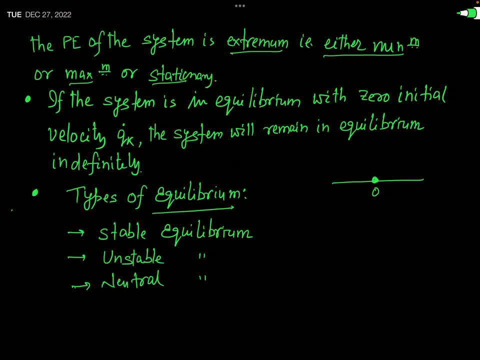 the potential energy function will be either minimum or maximum, or constant or stationary. Okay, Now, actually this equilibrium is of three types. The first one is known as a stable equilibrium, The second one is called unstable equilibrium and the last and third is called neutral equilibrium. 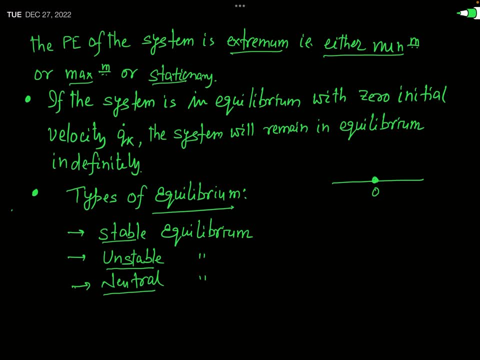 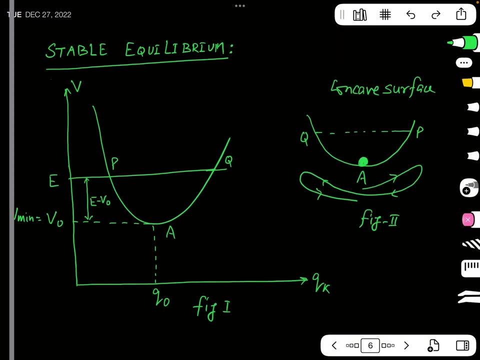 Okay, So we will understand what is this stable, unstable and neutral equilibrium separately. Okay, This is a very simple concept. you can easily understand it. So let us first of all see the idea of the stable equilibrium. In fact, for getting the idea of a stable equilibrium, let us consider that. see this figure two, this: 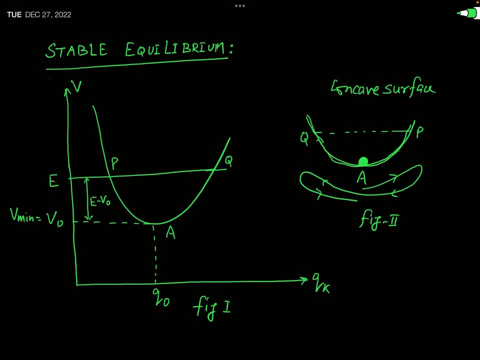 is just a vessel of concave state, Just like in Hindi you can say a Katora, okay. And at the lowest point of this vessel, let us consider, there is a system or there is a particle, which I have shown by this small sphere. 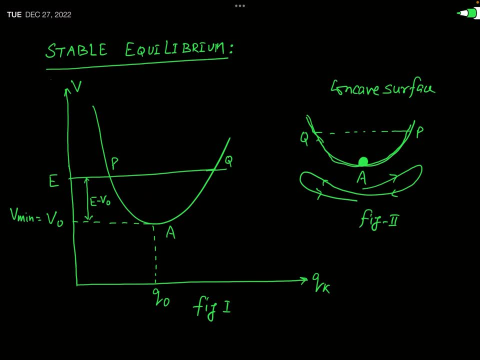 You can say by your experience that if this particle is at this lowest position and you watch the system at different times, you will find that this particle is at this lowest position. You will find that this system or this particle remains at that position A permanently. 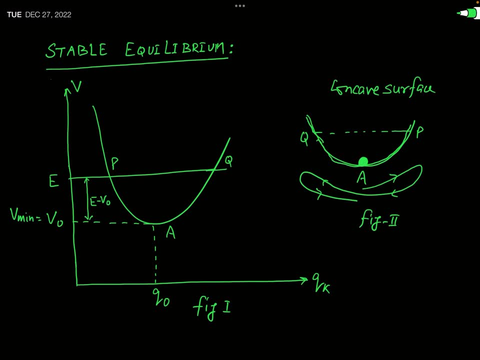 Okay, Now let us consider that this particle is slightly displaced to this position P, from the equilibrium, from this position A, and released. When the particle will be displaced from position A to P and released, then what will happen? You can say, Actually, this particle will back and reach to this point A, but, as you know, the particle 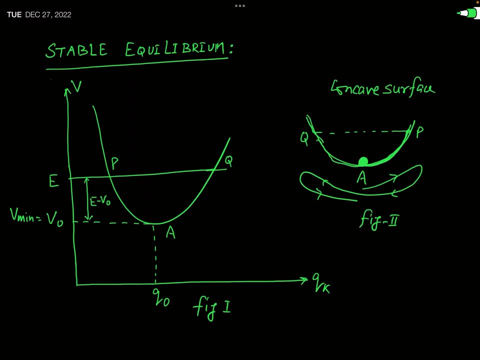 has mass. so due to inertia, it will shoot out in another direction and reach to the point Q, and when it will move from A to Q, its velocity will get decreased and reaching this point Q, its velocity will be again zero. Okay, Okay, So it will be again back to the position A. So in this way you can see that our particle 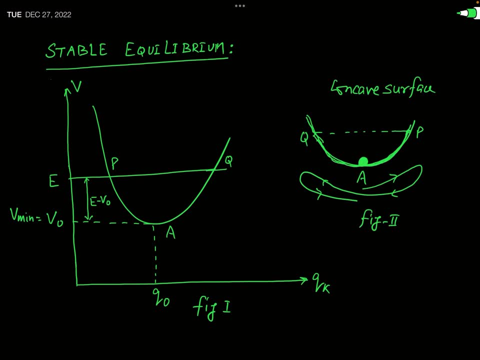 will in fact make motion about this point A, and whenever you will displace this particle from this position- A aside, slightly aside- then there will be a bounded motion, not unbounded. This type of motion is called a bounded motion. It means the part, as I have shown in this figure, the particle is displaced to the position. 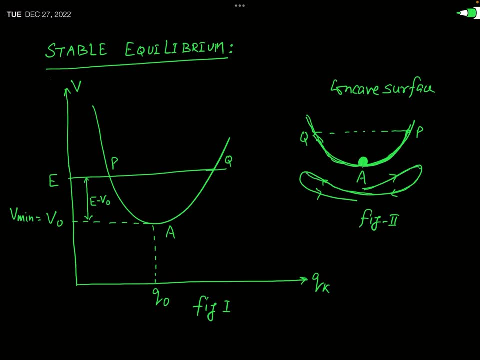 P and released, then it will come back and go in the another direction and again come back to A and again it will move to towards P, and so in this way, if a slight displacement is made from the position A, then the particle will perform a bounded motion. 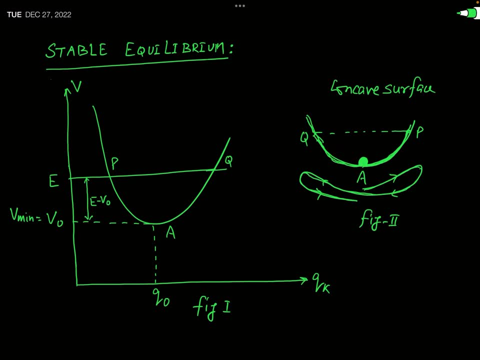 Okay, Okay. So in fact, if a particle performs a bounded motion about a particular point, that very point is actually the stable equilibrium position of the system. So you can say that this position A in figure 2 is the stable equilibrium position. Okay, 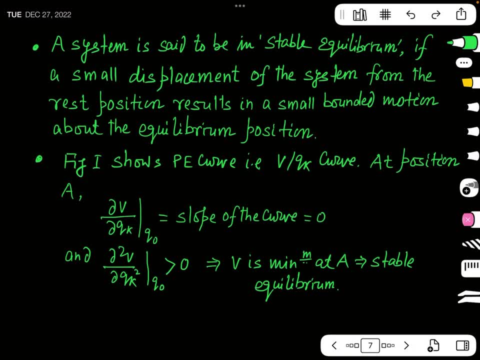 I have mentioned this fact here. you can see that a system is said to be in a stable equilibrium if a small displacement of the system- Okay, If a small displacement of the system from the rest position results in a small bounded motion about the equilibrium position. 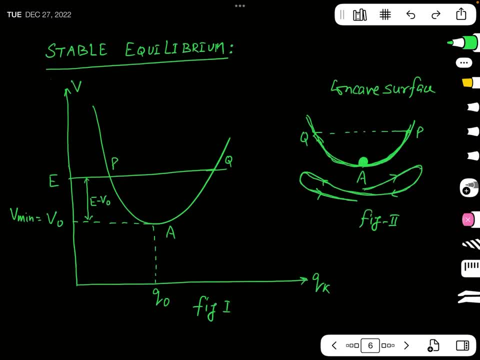 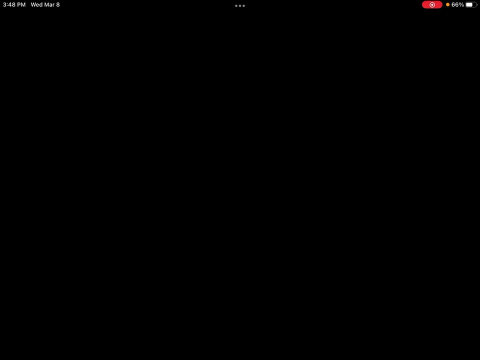 Okay, Now we can understand this concept of a stable equilibrium from this figure 1, where I have actually plotted the potential energy function V of the system in against of a particular value of generalized coordinate qk. So this is just a graph of potential energy function and the generalized coordinate qk. 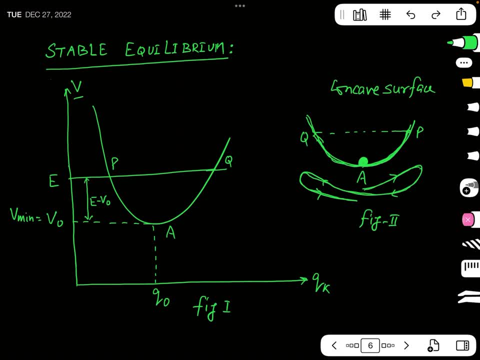 Let us see here: This is V versus qk graph. Okay, Actually, this graph which has been plotted between V and qk is called potential energy curve, And I have assumed it here. Okay, I have not given any potential energy function related to this qk. 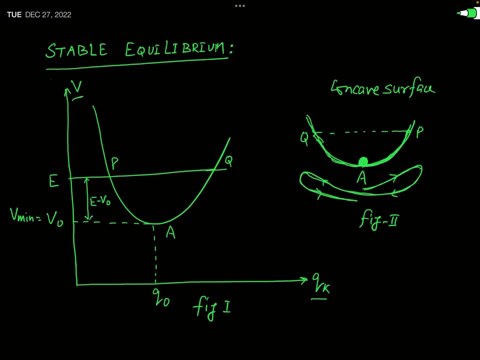 But let us say that if V is plotted in against of qk, we get a curve like this, which I have shown in this figure, and I am just marking this path. you can see. Okay, Now, this is just a potential energy curve, and if you see this figure, then you can find. 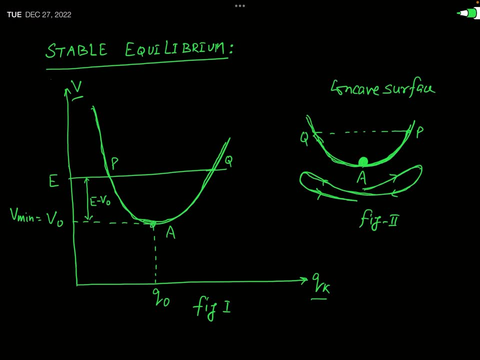 that corresponding to Point a, the potential energy function of this system is V naught and at any other point the potential energy is greater. It is greater than V naught. So you can say that potential energy function at point a, corresponding to point a, is minimum. 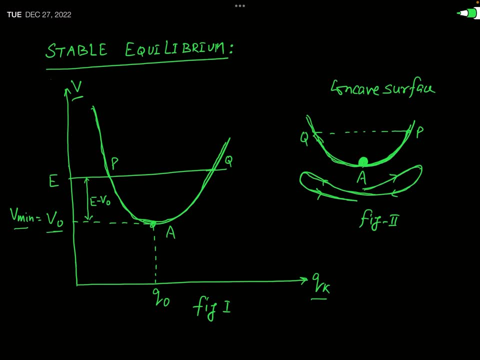 Okay, And you have the point corresponding, to which the potential energy function is minimum. At that point, the value of qk is q naught, Okay. In fact, at this point, when the system will be at this point, its potential energy will be minimum. 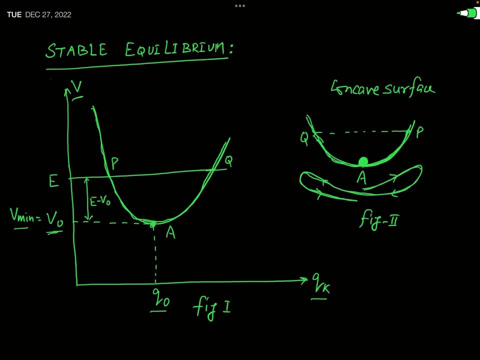 And this equilibrium minimum and this equilibrium position is called a stable equilibrium. This is called a stable equilibrium Because whenever the particle will be displaced- Okay- From this position, definitely its potential energy will increase and the kinetic energy will decrease. Okay, And if you let us take this particle at this position q, and its total energy is equal to: 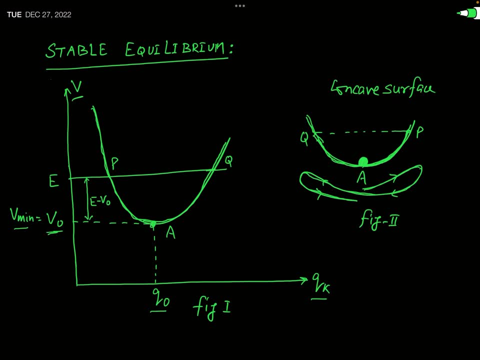 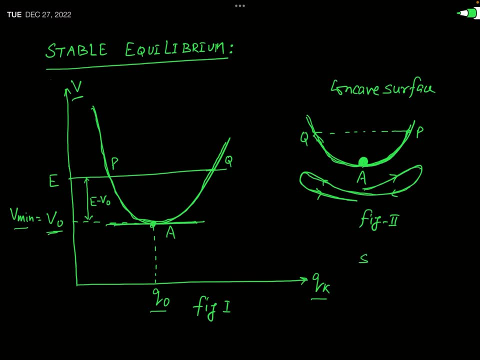 is parallel to the qk axis. it means slope of this curve corresponding to point a, which is equal to del v, by del qk at q, equal to q. naught, this will be equal to zero because it makes angle zero with qk and slope is equal to tan psi, where psi is the angle made by this tangent to the qk axis. 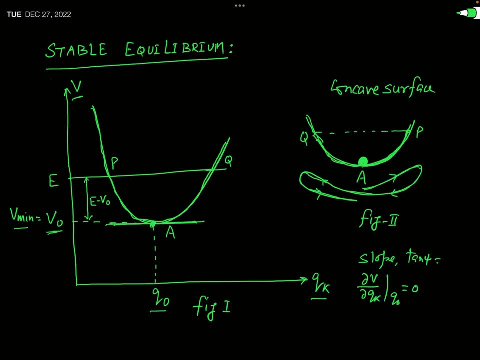 and this is actually zero, and tan psi and psi zero, so this will be equal to zero. so slope is zero. and it is also found that when we will take the second order, partial derivative, that is, del 2 v, by del qk, square del 2 v. 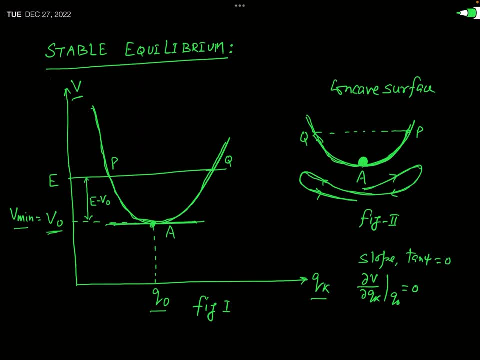 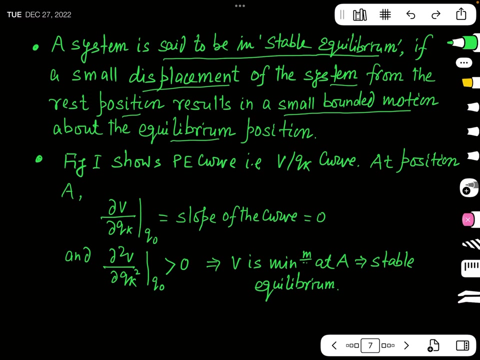 by del qk square, then this will be actually positive, because a small displacement from this position a increases the value of potential energy, and so this second order derivative will be positive. i have mentioned it here. you can see that at corresponding to point, a slope of the curve is equal to zero and the second order derivative is greater than zero. 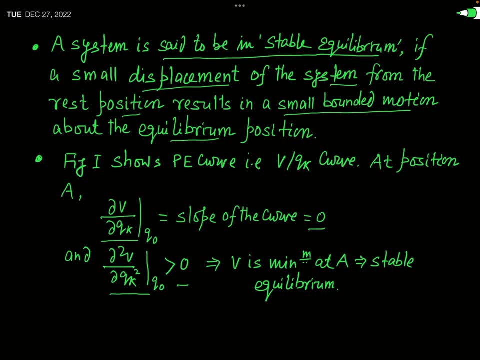 and if second order derivative is greater than zero. that means what you have definitely studied: the condition of maximum minima. in this condition you can say that v is minimum at corresponding to point a and this actually corresponds to the stable equilibrium. so you can say that if 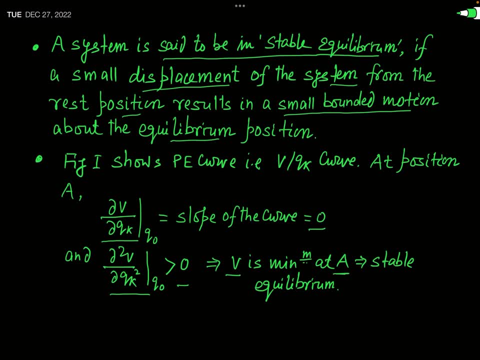 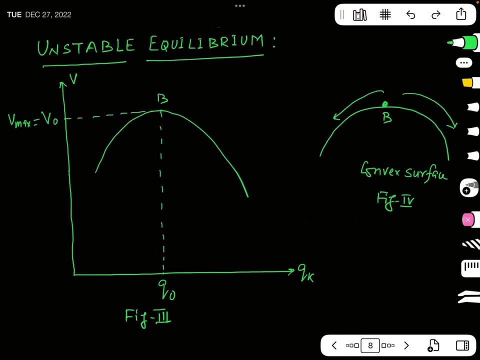 the potential energy function of a system is minimum at the equilibrium position, then we say that such a equilibrium position is a stable equilibrium. at a stable equilibrium position, the potential energy is minimum. okay, so i hope you have understand the idea of a stable equilibrium. now we will see the idea of unstable equilibrium. this is just reverse of that, for 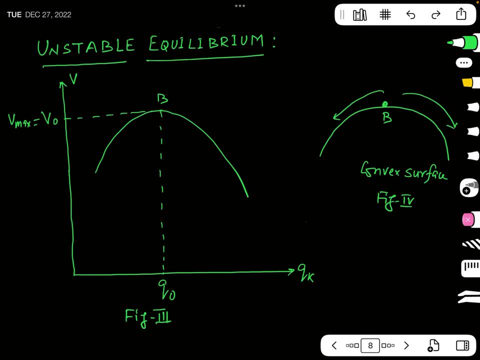 getting the idea of unstable equilibrium. let us now invert that katura, invert that pot, which is now in fact of convex, convex shape. so this is just a convex surface. you can say: and let us put a particle or a body or a system at its top position, it will remain in equilibrium, it will. 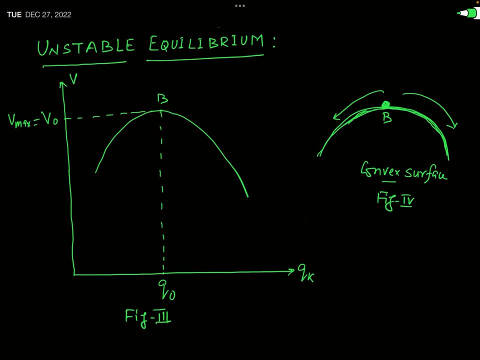 be a stationary. but imagine from your experience that if this particle will be displaced to this position and released, what will happen? this particle, when displaced from this position, be will not return back to be, but it will move away from B, and if you will displace this particle to this position, let us say C, then it again moves. 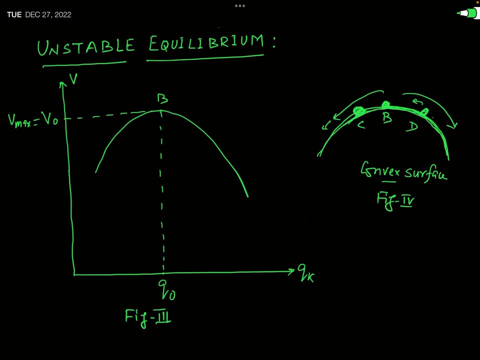 away from position B and never return, returns back to position a. this is called unbounded motion. so we simply say that a system is said to be in unstable equilibrium when the system is displaced from its equilibrium position slightly and the system performs unbounded motion, not bounded motion. about: 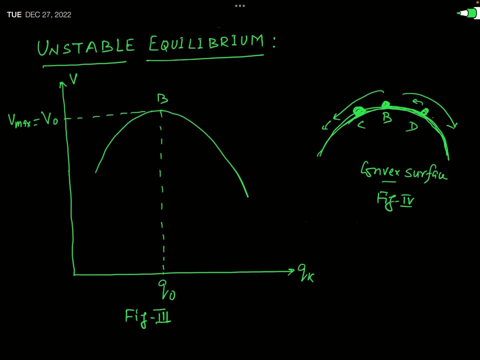 that point, then this equilibrium position is called unstable. okay, equilibrium position is called unstable. okay. now the same fact we will understand on the basis of this potential energy curve. here again, in this figure you can see we have shown a plot of potential energy function v in against of a particular value of the generalized coordinate a, k. 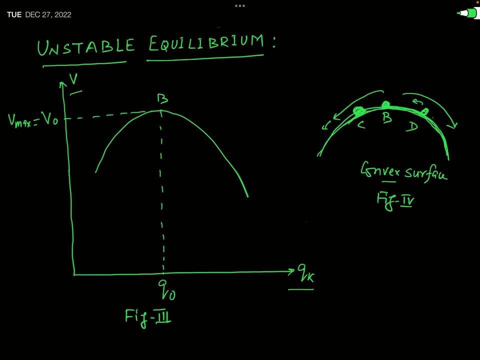 q, k. okay, and if the potential energy curve is like this shape, as which actually have shown in this figure, then you can see that, corresponding to this point b, the potential energy function is maximum, which I have denoted by the symbol v, naught. okay, and corresponding. 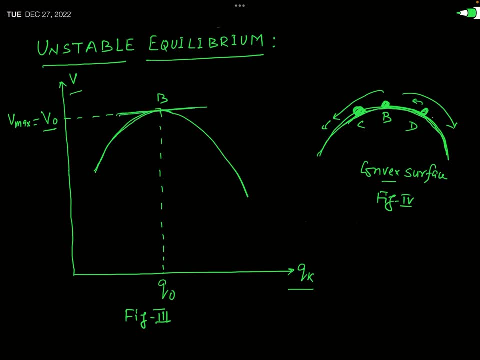 to this point. if you will want to find the slope of the curve, this will be again 0 for getting slope. what we will do, we will simply draw a tangent at this point B, and you can see that I have drawn here a tangent and this tangent is parallel to the Q- K axis. okay, and 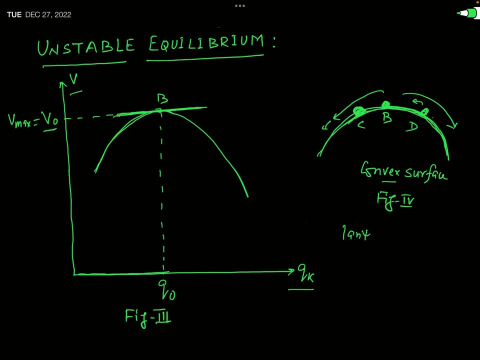 so the slope tan Psi will be again 0, because Psi is the angle made by this tangent with Q K axis, but it is parallel. so Psi is 0 and tan Psi is 0 and tan Psi. according to calculus this will be del V by del Q K, when Q K is equal to Q, naught see here corresponding to. 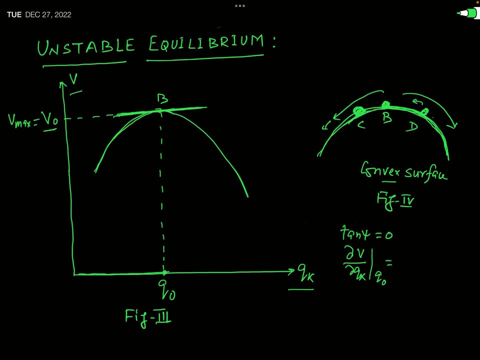 this point P, the value of Q K is Q naught and this is equal to 0. and at the same time you can see when you will find the second order derivative, that is, del 2 by del Psi 0, V by del Q K square. when Q is equal to Q naught, then it is found that this will be. 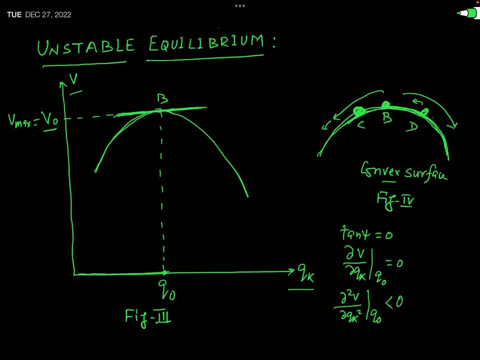 a less than 0, that is negative. and if it is negative, according to calculus, according to the condition of maxima, this potential energy function will be maximum. so this point B corresponds to the maximum potential energy of this function and this also corresponds to the unstable equilibrium. so in one sentence you can say: 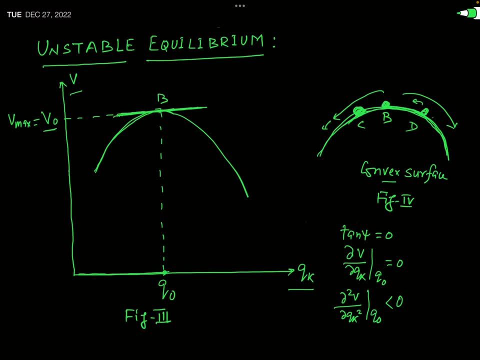 that the state of the system when it's potential energy function is maximum, that is called unstable equilibrium state, okay. when B is maximum, that is called unstable equilibrium state. when B was minimum, that was stable equilibrium state, ok. and when d is maximum, that is unstable equilibrium state. 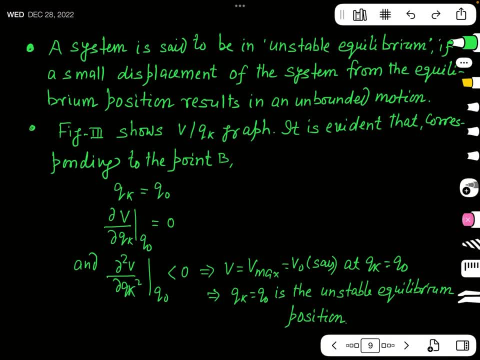 And all these things which I have just explained that are here mentioned. for your convenience, you can note down these things in your notebook. you can see that I have mentioned that a system is said to be in unstable equilibrium if a small displacement of the system from the 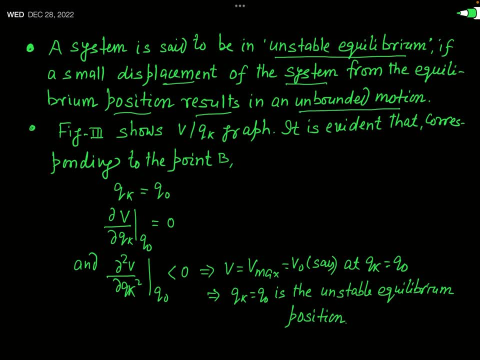 equilibrium position results in an unbounded motion. mark it unbounded motion and according to the v versus k graph, it is evident that the corresponding to the point b, that is q k equal to q naught, del v by del q k at q naught is zero and del 2 v del q k square. 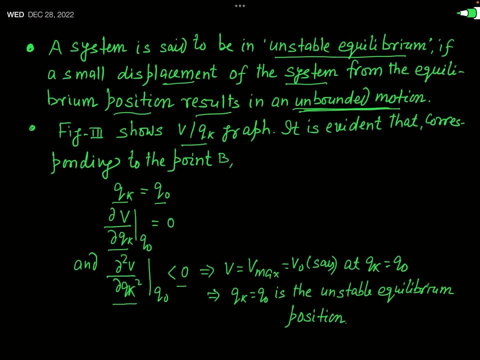 at q naught is less than zero, And if it is less than zero then it is equal to 0.. v will be v max, which I have assumed. v naught at this position q naught, and so this implies that q k equal to q naught. this is the unstable equilibrium position of our system. okay. 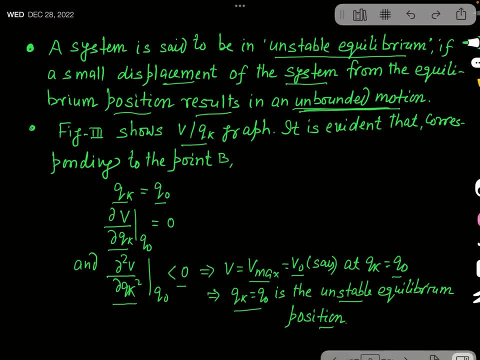 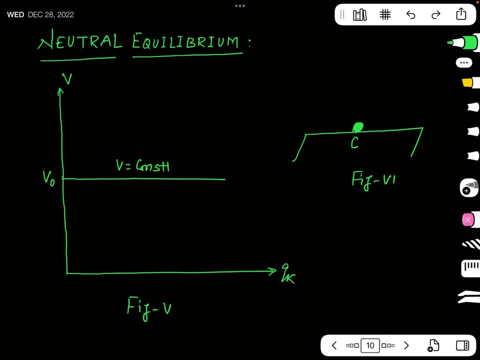 So I hope you have understand the concept of this unstable equilibrium. okay, Now the third one, which is called neutral equilibrium. For getting the idea of neutral equilibrium, let us consider now: there is a plane surface. you can see, this is a plane surface, okay, just like surface of your table. and at that plane, 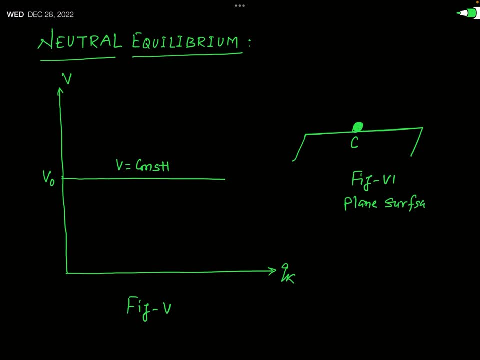 surface at any point c. let us consider there is a small sphere or any particle or any system placed. Now let us displace this particle from this position c. So this is the plane surface. This is the plane surface At c. the particle is at rest, it is in equilibrium and we simply provide a small displacement. 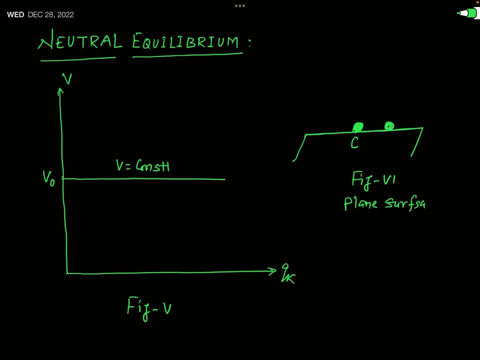 to this particle on this horizontal or this plane surface, Let us say it is displaced to the position d, What will happen? You can easily say from your experience that if the surface is horizontal, it is plane. then, after displacing the system from this equilibrium position c to d, 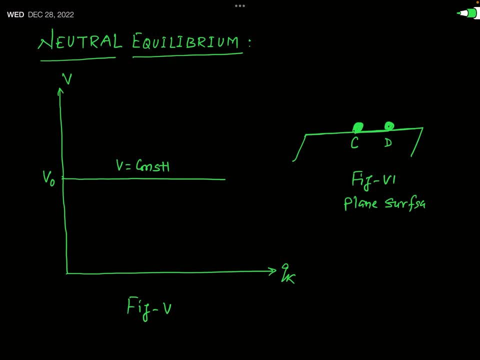 So that is the plane surface. Again, this particle will remain in equilibrium. It will neither move towards sea nor away from sea. It means this particle will neither perform a bounded motion nor an unbounded motion. It will perform no motion. Similarly, if you displace the particle at this position E even then you find that the 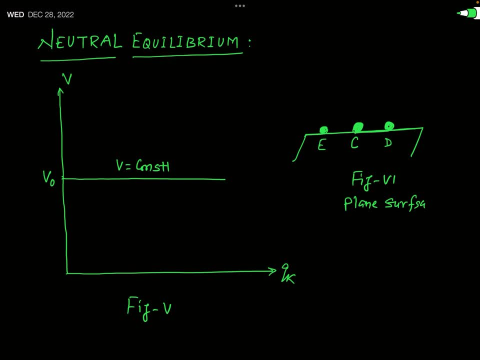 particle will again remain at rest. So you can say that if a system is in a neutral equilibrium, what will happen Then? after providing a small displacement from the equilibrium position, then the particle will not execute any type of motion. The particle will be again in equilibrium position. 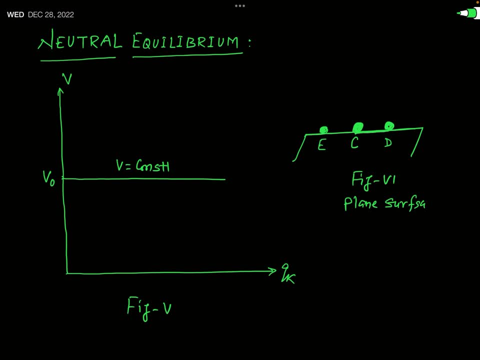 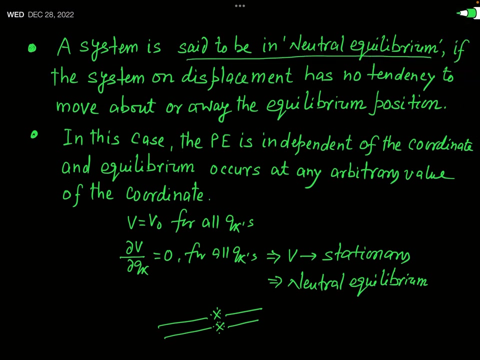 So this is So. in this condition, You can say that this point C or D or E, all are actually the position of neutral equilibrium. Okay, In fact I have mentioned it here. You can see that a system is said to be in neutral equilibrium if the system on displacement. 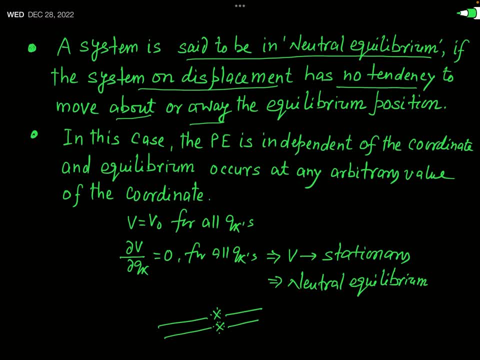 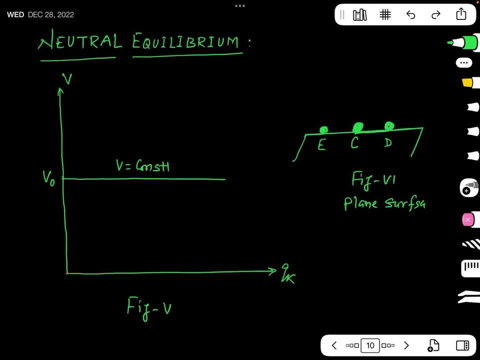 has no tendency to move about or away. the equilibrium position. Okay. So such an equilibrium position is called neutral equilibrium position. Now see this figure five where I have plotted the potential energy function in against of QK. That is generalized coordinate. In fact, if the system is in neutral equilibrium, its potential energy function is completely. 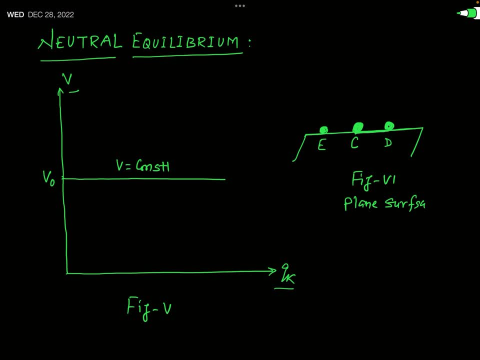 independent of position. You can see here the potential energy of the system at point C and at point D, at point E. everywhere is same, So the potential energy function does not change with change in position. Okay, So you can say that if the system is in neutral equilibrium, its potential energy will be. 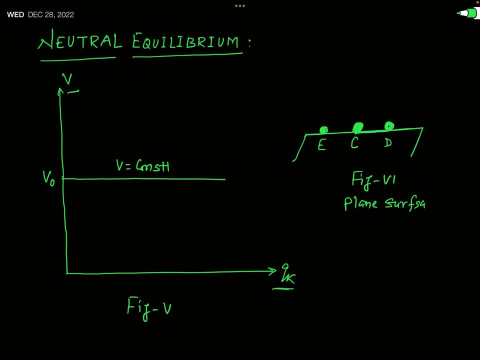 independent of generalized coordinate or independent of position. So when QK is zero, then V is equal to V. naught, When QK is, let us say this much Again, You can see that When QK is equal to, let us say this much, let us say QK is here Q1, here it is Q2.. 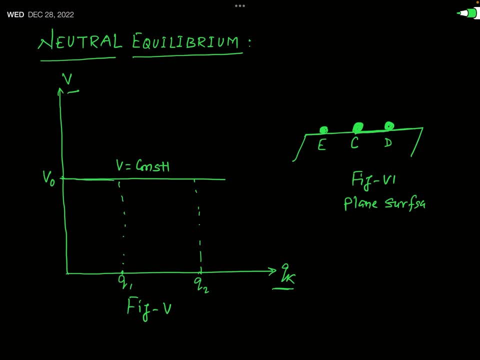 At for all values of QK. you see that V does not change, It remains constant, And so this curve is just parallel to QK. Okay, Just parallel to QK. And since it is parallel to QK, So the slope at any point on this curve. 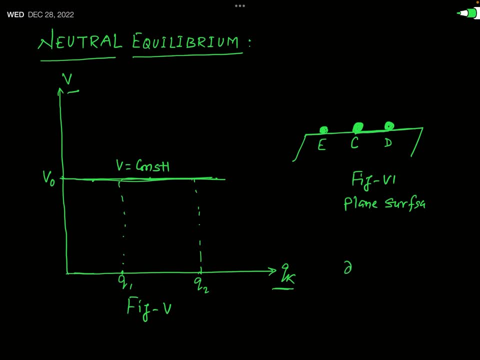 Okay, At on this curve will be equal to zero. Okay, Del V by del QK, at any QK will be equal to zero, And in that condition we say that our system is in neutral equilibrium. So main fact is that in neutral equilibrium potential energy function is stationary. 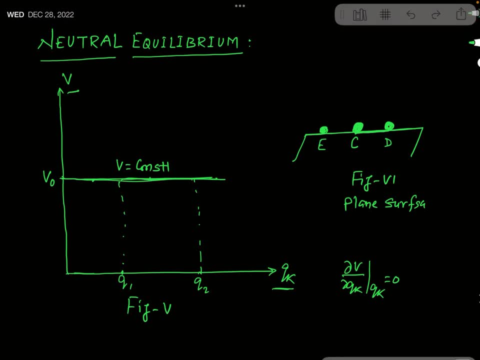 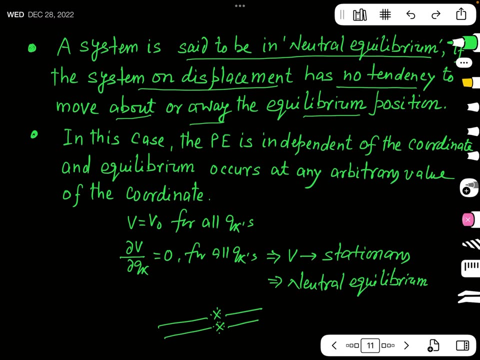 It is constant, It is independent of position. Even after, Okay, After a displacement from the equilibrium position, potential energy function does not change. So I have mentioned it here. You can say that in this case the potential energy is independent of the coordinate and 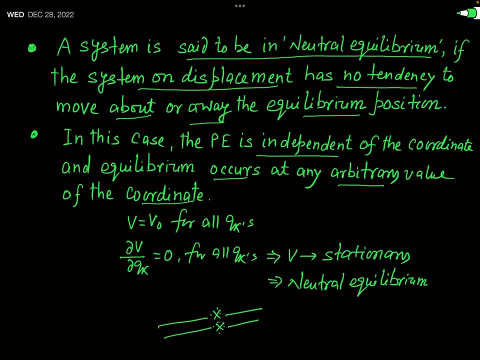 equilibrium occurs at any arbitrary value of the coordinate. So V equal to V naught for all QKs, and del V by del QK, equal to zero for all QKs. Okay And So, And you can see, this is a stationary. 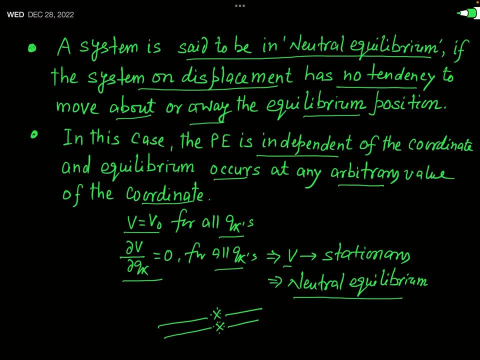 A stationary means constant, And this represents actually the neutral equilibrium. Okay, So these three types of equilibrium, I hope you have understand. but what you think when you talk about the oscillation or vibration of a system, about an equilibrium position, about which equilibrium position, vibration will take place? 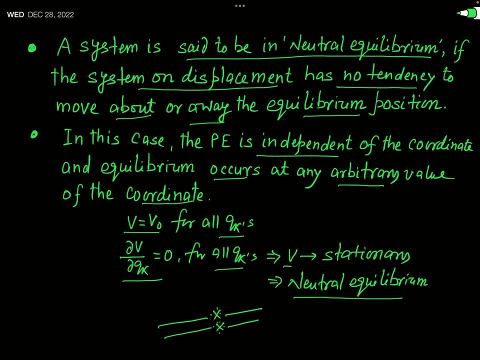 Can you say Definitely? You have seen that case of a stable equilibrium. the particle performs a bounded motion about the equilibrium position. so definitely, when we talk about the oscillatory motion or vibratory motion, that motion always takes place about the stable equilibrium position. vibration will not take place about the neutral.